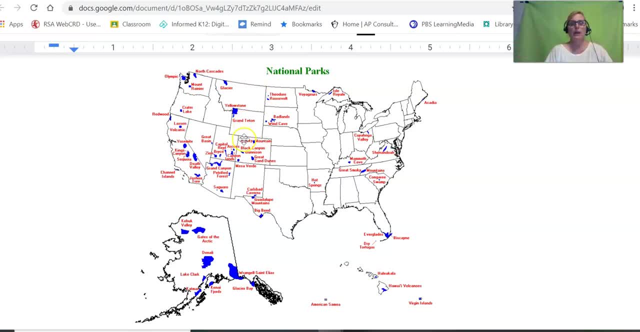 country. there's some beautiful places, wildlife, painters and photographers would go over here, take pictures, send them back east and go look at what's here. we need to save it, and so they created national parks. the first one was created in the 1880s, which was yellowstone, but they really 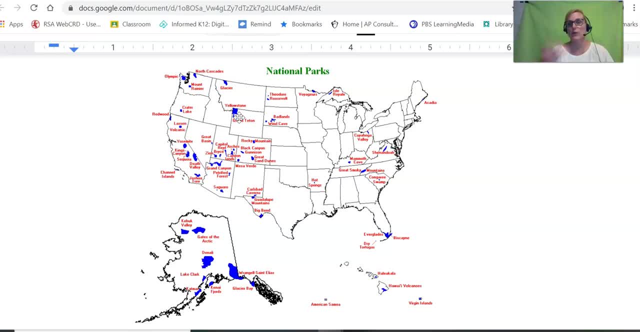 got a big ramp of the number of. they saved a ramp up in the early 1900s- think teddy roosevelt was a big part of that- and so most of the land that was not sold off or given away to settlers was in the 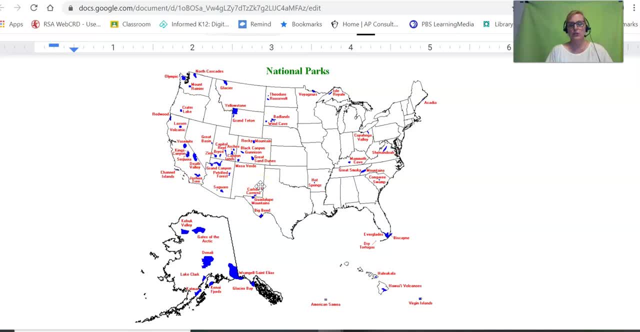 western united states. so the reason why we have most of the national parks in the united states was because the land that was left to save happened to be more in the west than the east, which was already settled. so we're very, very lucky here in california that we 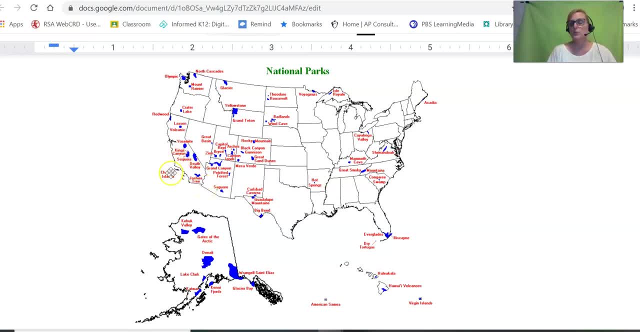 have about 10 national parks within a day's drive. you can get to sequoia in four hours, king's canyon and, you know, four and a half, yosemite in about six hours. you can get to the channel islands in about an hour drive to the coast and then about an hour and a half boat ride. 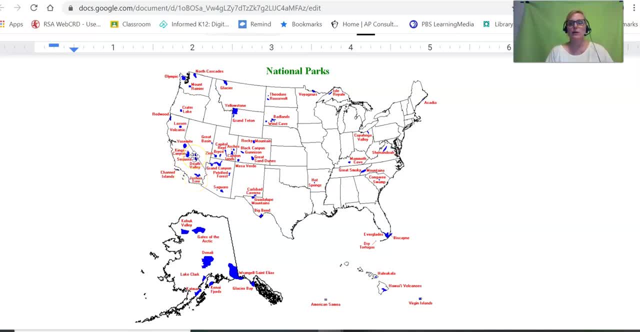 joshua trees about three hours south and then about an hour and a half south, and then about death valley is about four hours north, in east zions about a seven hour drive. grand canyon is about a six hour drive so, and bryce is maybe an eight hour drive, so we're really, really lucky. 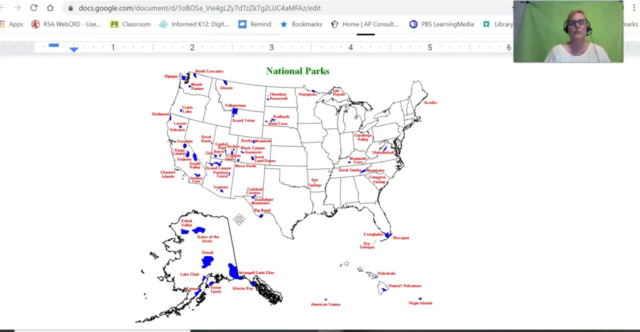 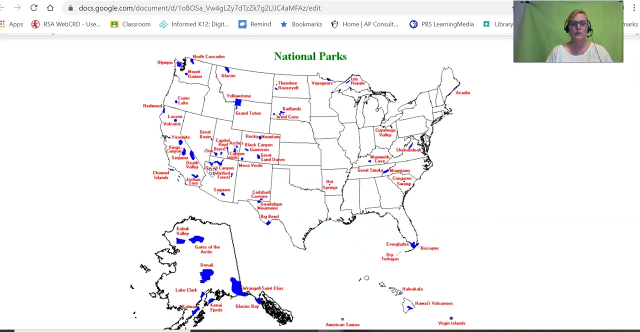 that we have so many national parks that we can drive to in a day, all right. so this theory of island biogeography theory, which of these national parks would have the most national parks, the most biodiversity? think about it for a minute. I hope you said the big ones. 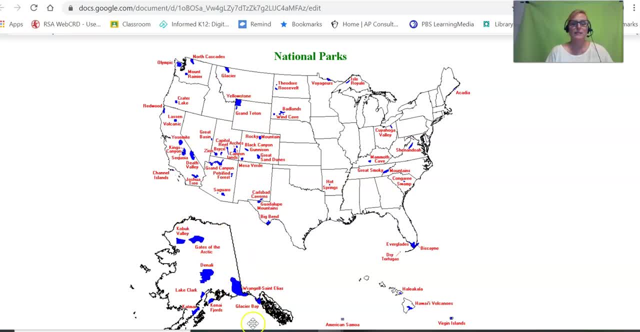 Yellowstone. up here in Alaska are some very big ones- Denali, Wrangell, st Elias- but what about the smaller ones that are clumped together? in Utah you have Capitol, Reef, Arches, Bryce, Zion Canyon lands. they're smaller but they're clumped, so that kind of refers to the distance up from the mainland right. 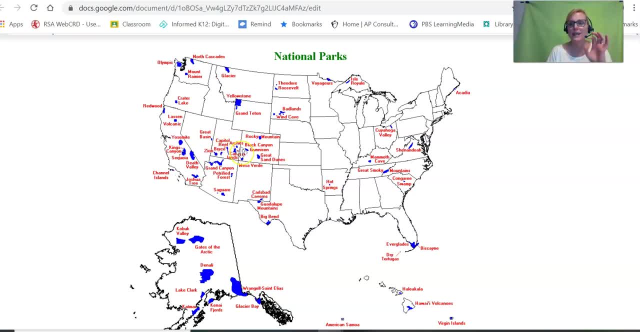 these are not real islands in the ocean. these are islands of habitat on the continent. what about up here? we have kind of a clump in the Cascade Mountains, North Cascades, Mount Rainier, Olympic- I've been to all three went to Mount Rainier to about a year and a half ago. it was absolutely amazing. 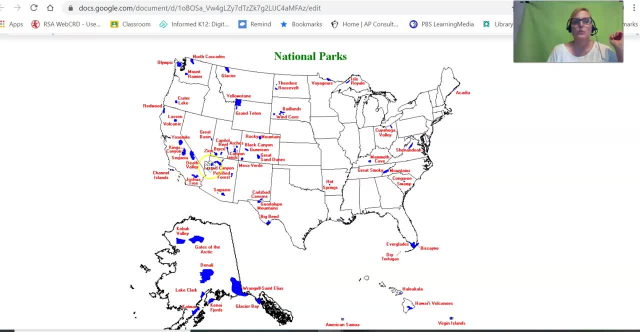 I'm going to show you some of the other islands that are clumped together in the area, so the smaller ones that are close together- even here it's Yosemite, Kings Canyon, Sequoia- they're going to be close enough that your species can go between them. a lot of species, not all, but a lot of species can go between them. so 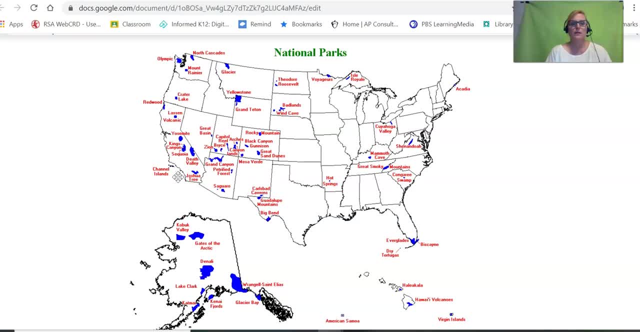 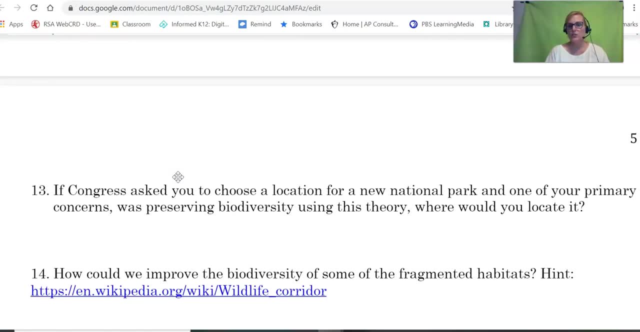 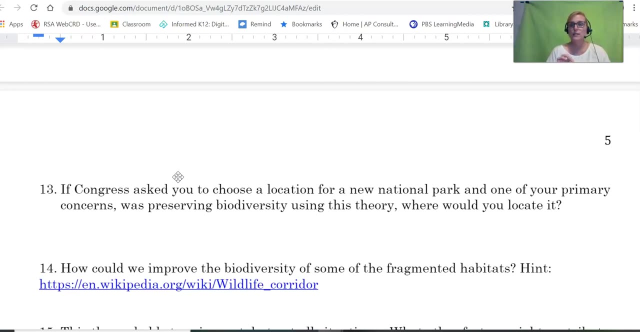 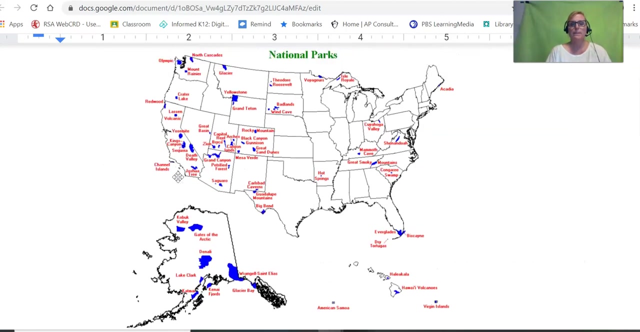 they're going to have more biodiversity. the next question, number 13: if Congress asked you to choose a location for a new national park and one primary community, would you choose? if your primary concern was preserving biodiversity? with this theory, where would you locate it? so, just based on this theory, let's talk about some other. 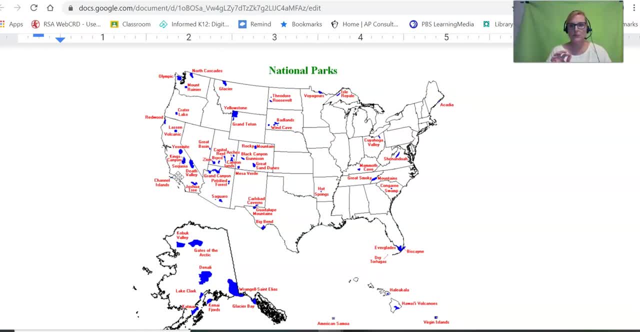 answers that aren't based on the theory, so don't write them down. a lot of students will say we need to have one in the middle of the United States because they don't have one there and we need to protect the species in the middle of the. 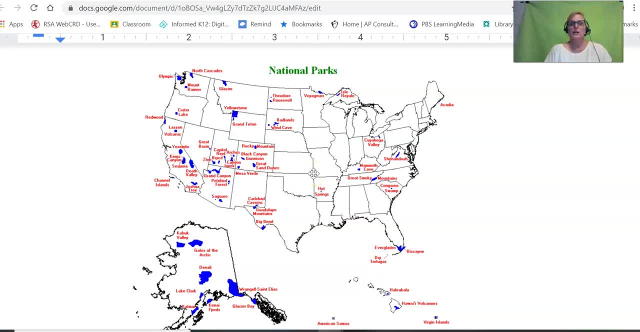 United States, Kansas, Nebraska. yes, that's a good idea, but it's not the correct answer for this question, because it there's nothing, there's no big ones that surround it, so you're going to have very limited biodiversity, even if you protect the land, are going to have very 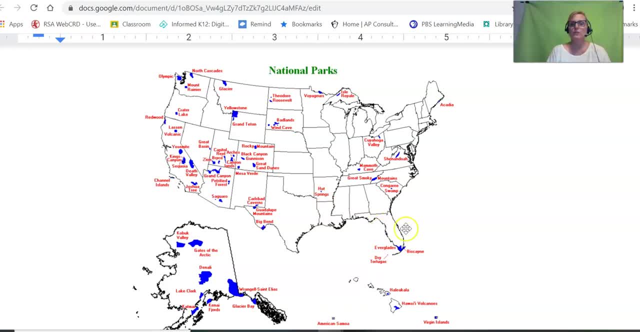 limited biodiversity. sometimes students say, well down in Florida because it's tropical or sub-tropical and there that usually means more biodiversity of species. that is also true that there are is more biodiversity in subtropical and tropical regions, and if you place that National Park right down here next to the Everglades and Biscayne, that would make 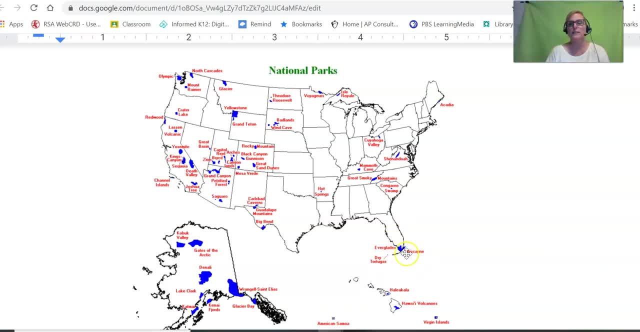 sense, so that might be an okay, as long as you placed it next to the others. what if you said the Channel Islands because of endemic species? so yes, there is a lot of endemic species at the challenge Channel Islands National Park, like the Channel Islands Fox is one, so that is a good place to preserve species. 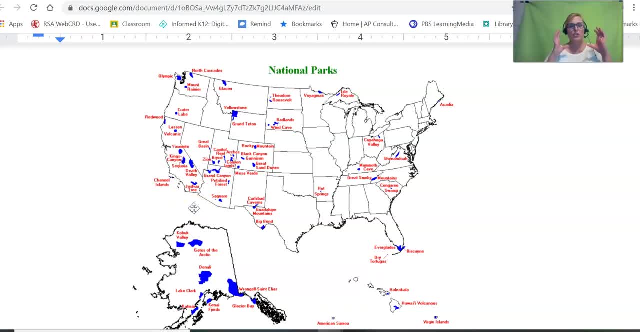 but if we are focusing our question just on this theory and preserving and really upping the number of species, where would you place it? you'd want to place it next to other big ones, so maybe over here in California in this cluster of kind of big ones- not that big but kind of big- national parks, Yosemite. 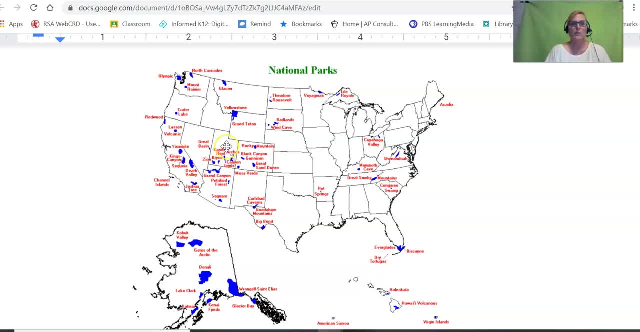 Kings Canyon, Sequoia, Death Valley, maybe here next to Yosemite, I'm sorry- Yellowstone and Grand Tetons. on a side note, did you know they're trying to buy land to connect glacier and Yellowstone National Parks so that the species- they're like the grizzly bears- can travel between safely. right now it's. 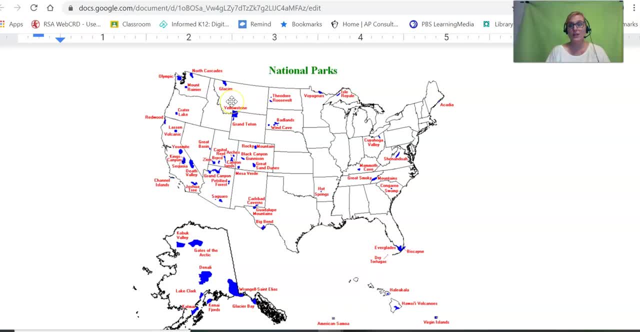 private land with ranchers and and they're- they're cattle and they don't want grizzly bears roaming between those two national parks. there's, there's grizzly bears in very few places left in the whole United States. they used to roam California shores. is not amazing, but they were hunted to extinction in. 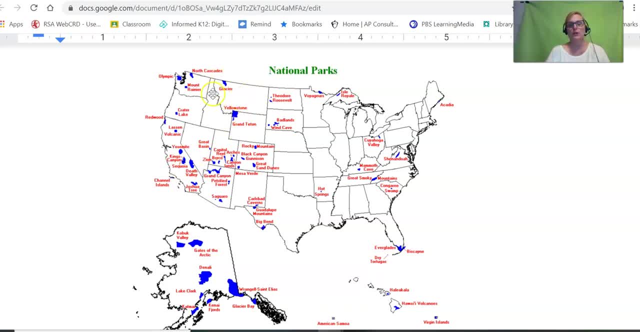 most states, except for in this area, is called a greater Yellowstone area ecosystem. anyway there's land groups trying to buy land to connect glacier Glacier National Parks with Yellowstone, So those two grizzly bear populations can travel and breed and prevent bottleneck effect for species And up into Canada too, because there's grizzlies in Canada. 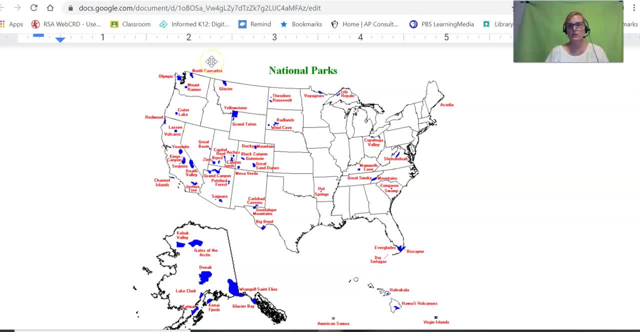 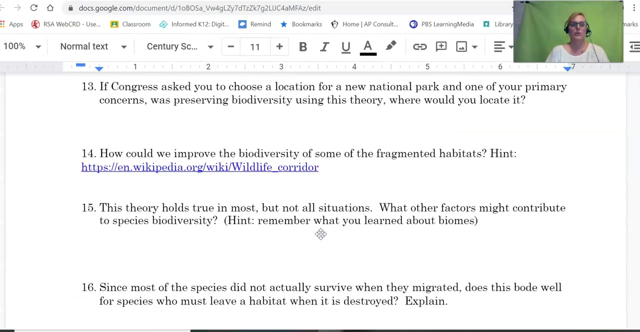 So there's more national parks up in Canada that they want to connect as well. It's called a wildlife corridor. It's not done yet, but they're working on it, Or another national park in Alaska near these other large national parks. So those are the best answers for number 13.. 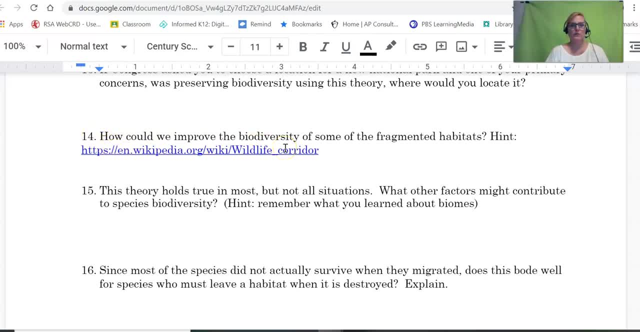 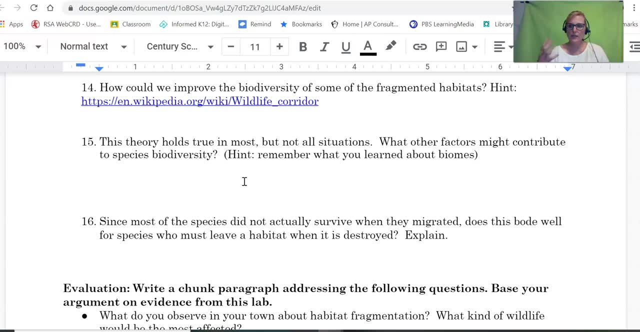 Number 14 asks you to look at wildlife corridors. Number 15, now you can think about other things that are important to you, Things that influence biodiversity, like tropical regions. So that's latitude near the equator: The more water there is, the more endemic species there are.